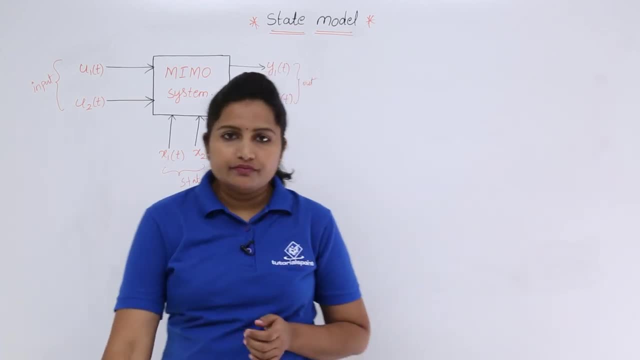 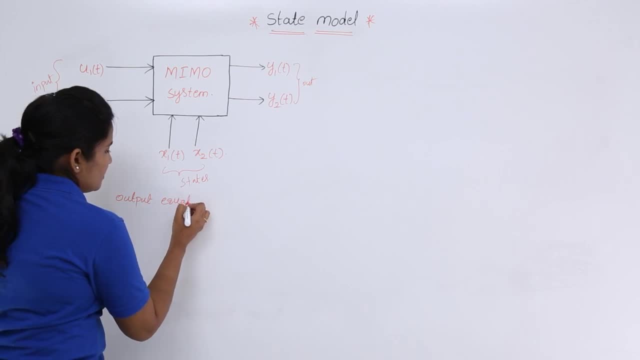 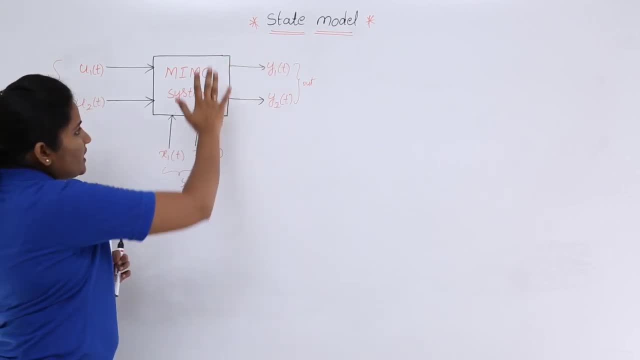 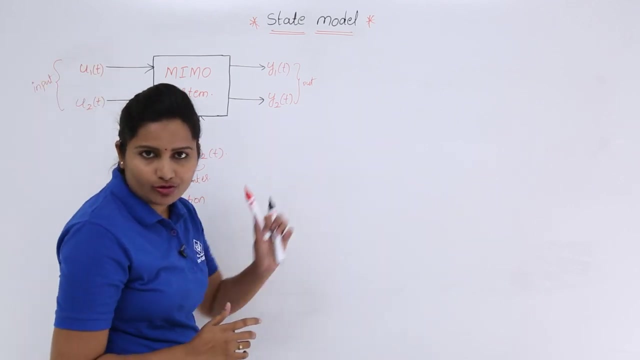 for this output variables. So the inputs for the system are two inputs and two state variables. So which gives the past history? this state variables will give you the past history. by taking this past history and with its present input, we need to get the output. 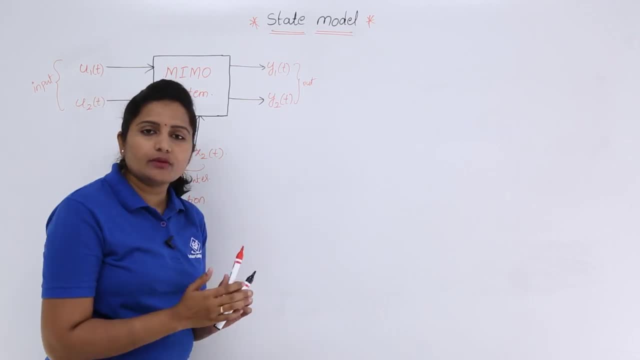 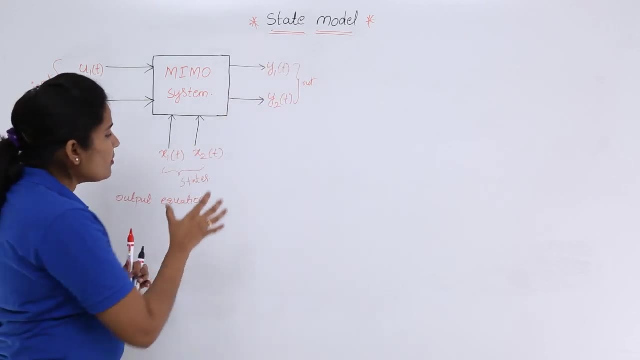 for this M I M O system. So which gives the past history, this state variables will give you the pi죠 system and we will get the I M G I M A M O system. So here, when we are creating a condition, which relates to A or puts M 1 of X Levi time, we need to write As sin holistic V shape of M. So the variable means multi output system. So here, definitely, this output will be in the form of this state variables and this input. So here, when we are writing or when we are equating any variables with any number of variables, any other number of variables, definitely we require a coefficient And恤. 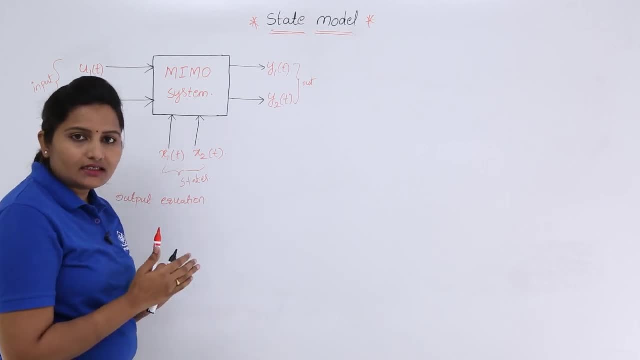 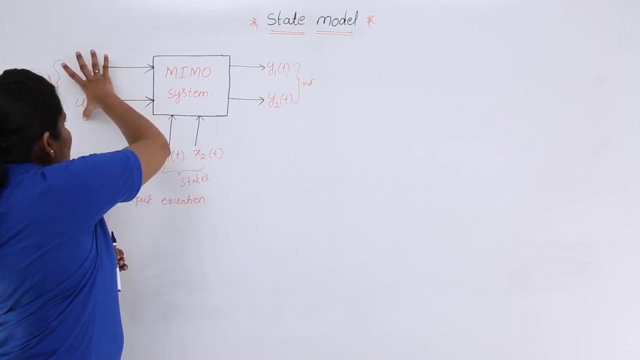 That coefficients I am considering here as c and d. When I am writing, when I am writing state variables, I will consider c with some suffix and I am writing u, that means input variables. I used to take d for your reference. And here I am start. I am going to start y. 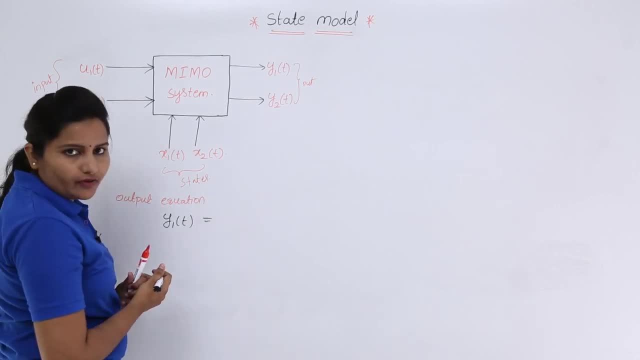 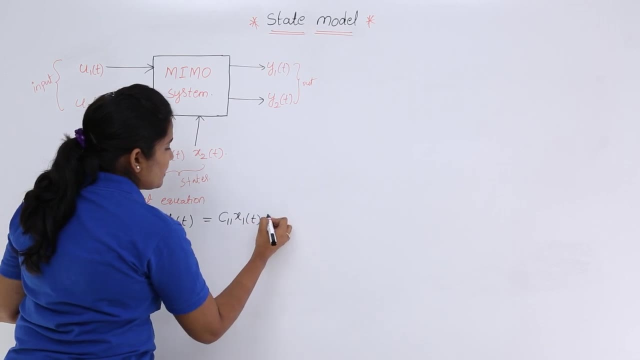 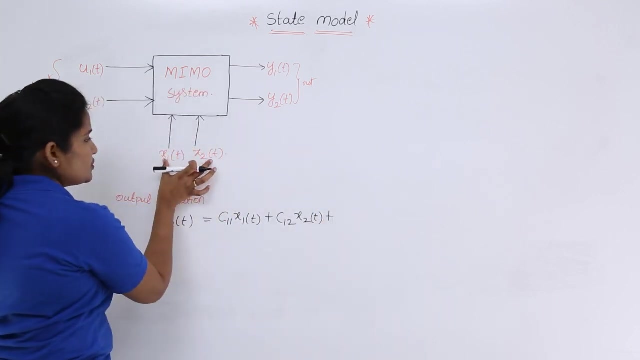 1 of t. if I want to write y 1 of t, y 1 of t is equivalent to c 1: 1 x 1 of t plus c 1, 2 x 2 of t plus. So these two are over with the coefficients c 1: 1 and c 1: 2.. As I told, 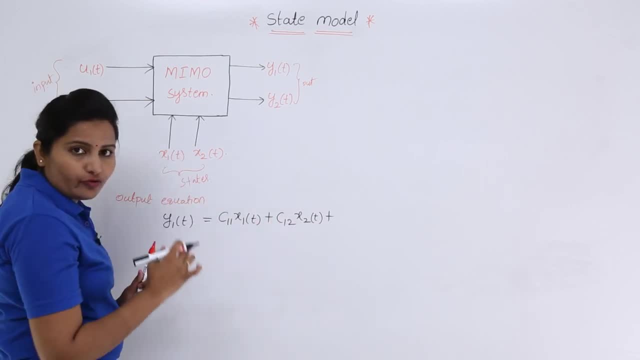 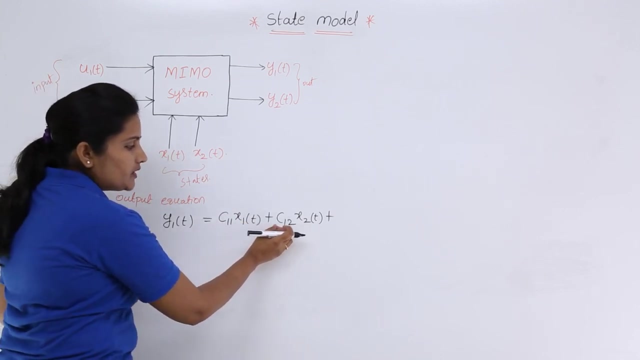 you. I am going to take c as my coefficient when I am writing x 1 and x 2 in my output equation. So my output variable y 1 of t can be determined by using this state variables and input variables as c 1, 1 x 1 of t plus c 1, 2 x 2 of t. 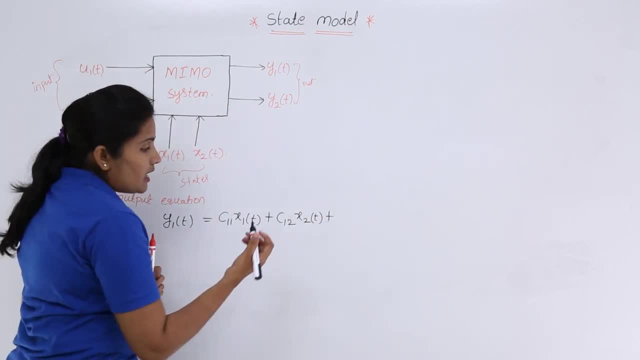 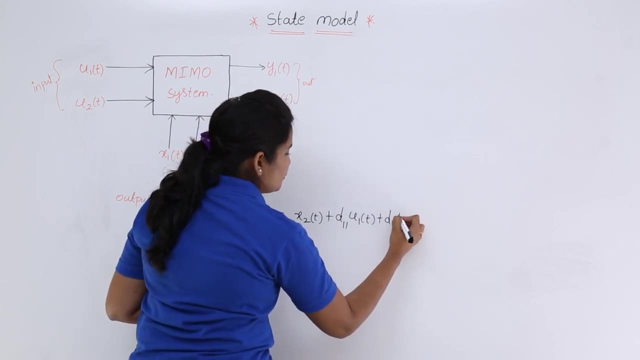 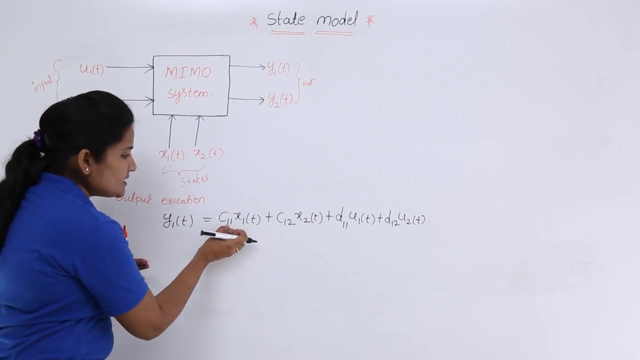 When I am writing this input variables, I am going to consider d, d, 1, 1 u, 1 of t plus d 1, 2 u, 2 of t. So I written equation for this: y, 1 of t. Similarly why I consider 1 ever. 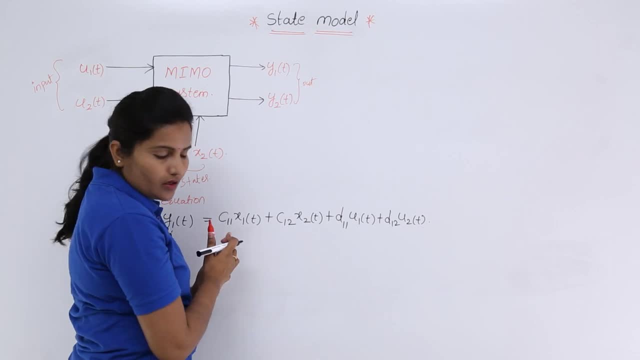 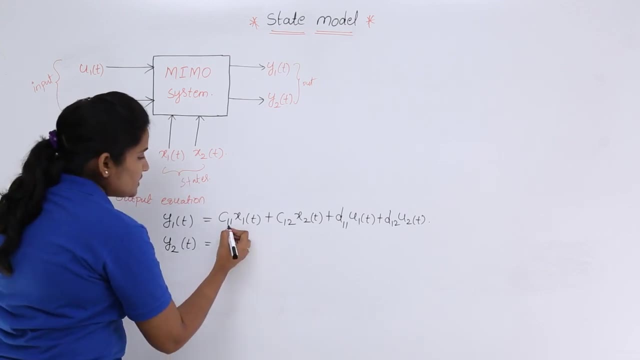 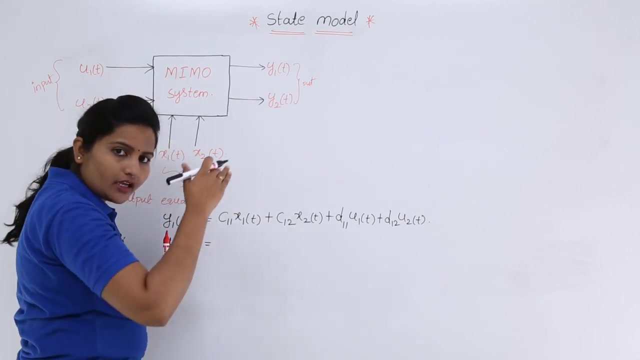 where means to refer y 1.. So like that, if I want to consider y 2 of t similarly, I am going to consider same these two state variables. that means another output variable, y 2 of t also came from these variables. So that is why in that output equation also you are. 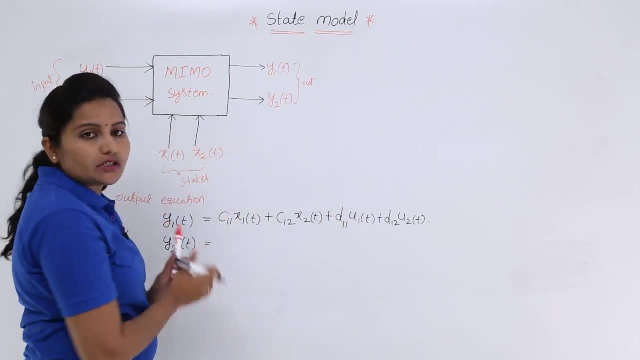 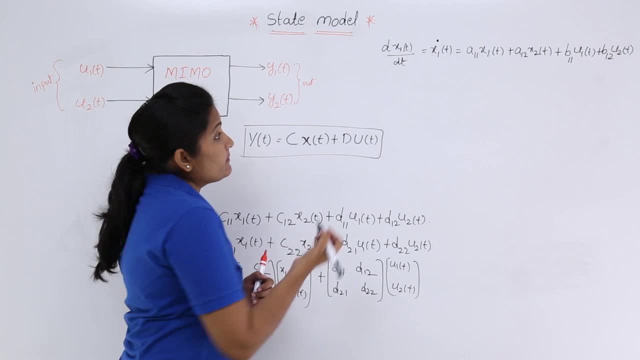 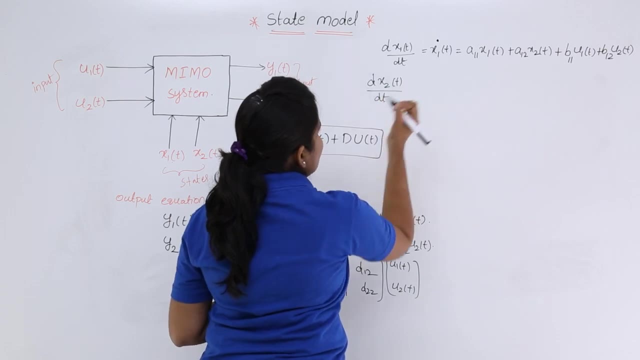 So that is why in that output equation also you are having samples of that variables. Now, similarly, when you are writing the equation for second state variable, x2 of t, differentiation of second state variable. So this I am considering like x2 dot of t. 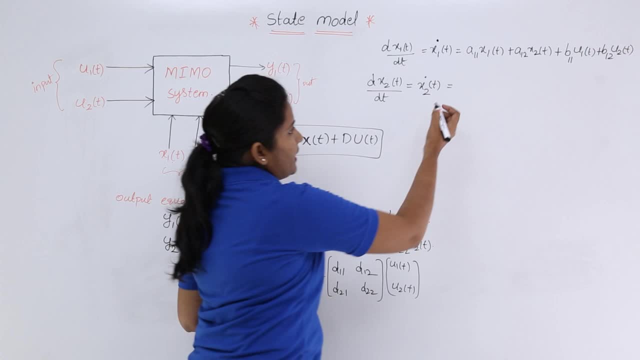 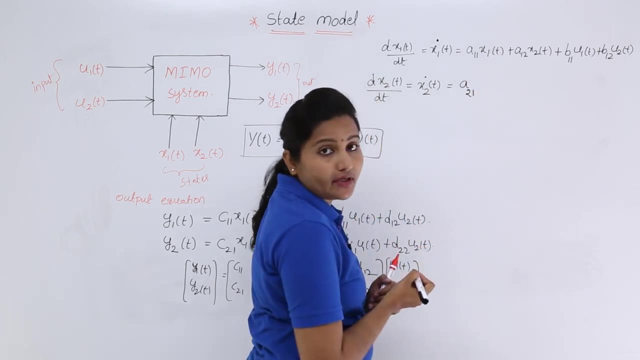 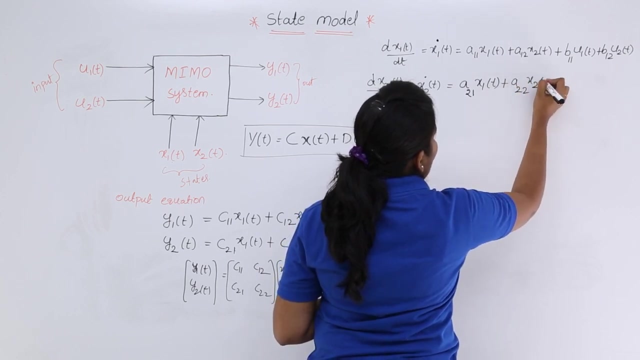 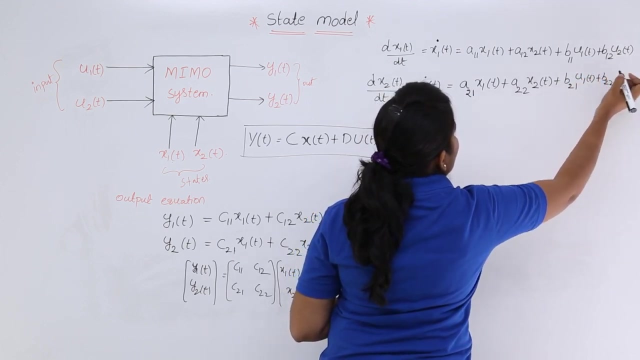 So this is equivalent to: again you are writing for second state variable. So that is why a21 with first state variable, a21 into x1 of t plus x2 of t, A22 into X2 of T plus B21, U1 of T plus B22 into U2 of T, As we written here in the matrix form. 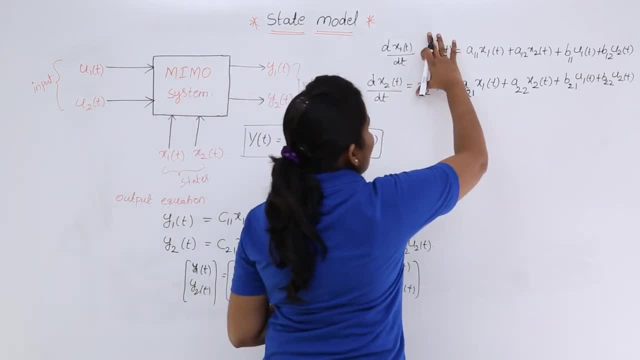 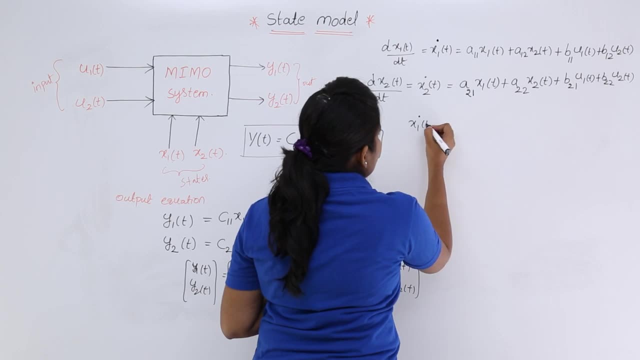 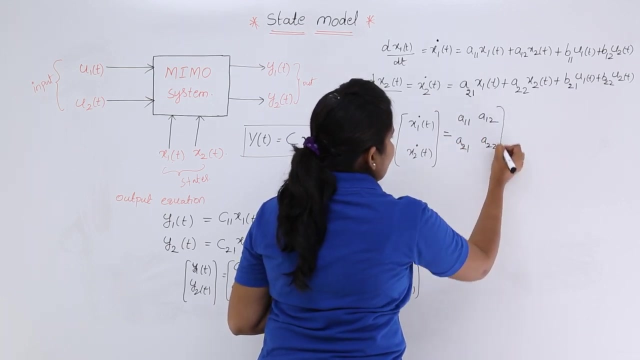 here also we can write in matrix form These two. I am considering this complex to write, So that is why I am considering like this: X1 dot of T, X2 dot of T. that means differentiation of X1 of T and X2 of T is equivalent to A11, A12, A1, A21, A22.. This is one matrix and another. 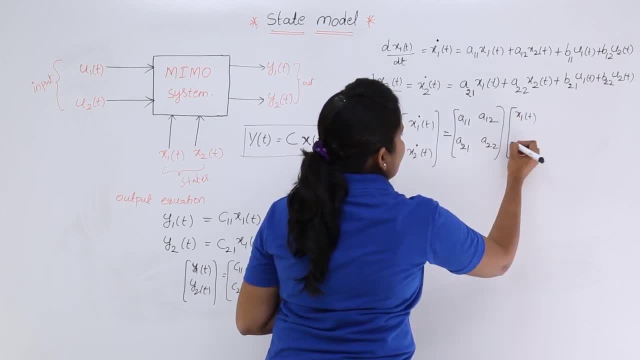 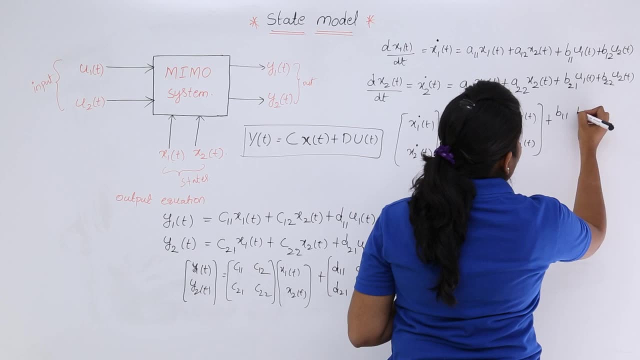 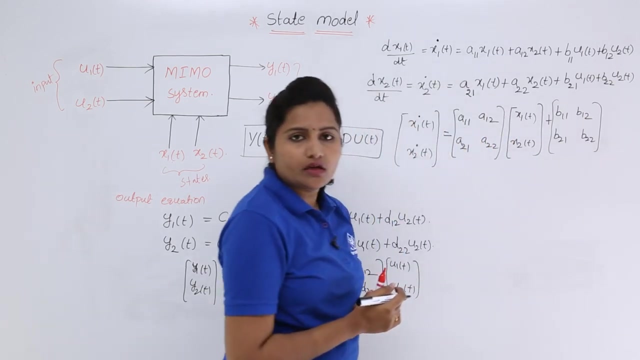 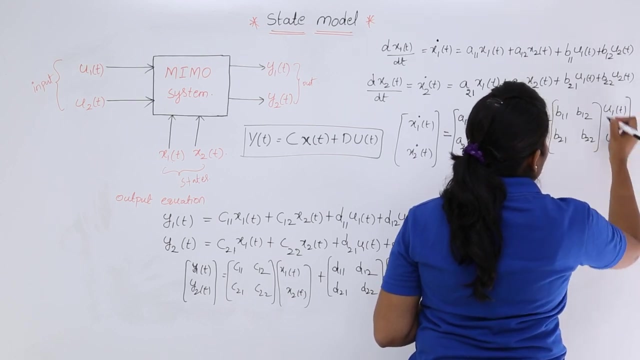 matrix is X1 of T and X2 of T. Now place B11, B12, B21, B22 into this one matrix And here you are having another matrix that is U1 of T into U2 of T, If you observe, if 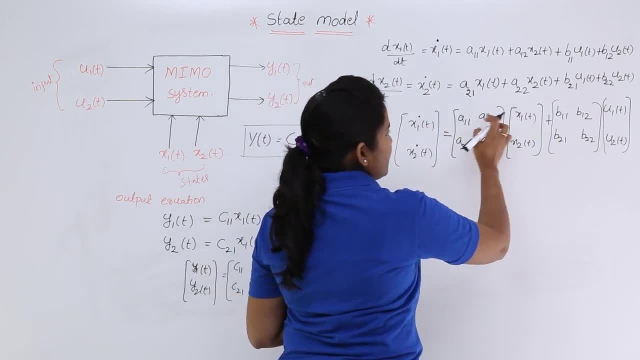 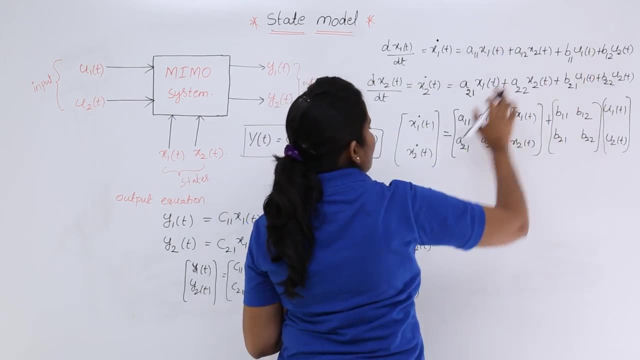 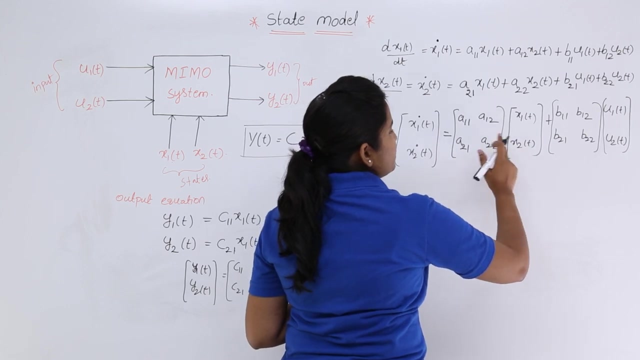 you want X1 dot of T, A11 X1 plus A12 X2, B11 U1 plus B12 U2.. So this four will come If you want this one. So you will get A21 X1 plus A22 X2, A21, B11, B21 U1 plus B22 X2.. So 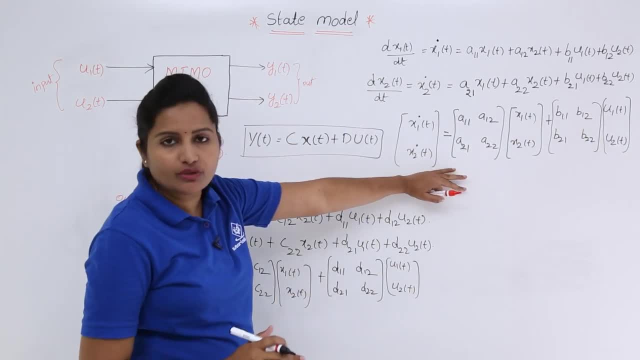 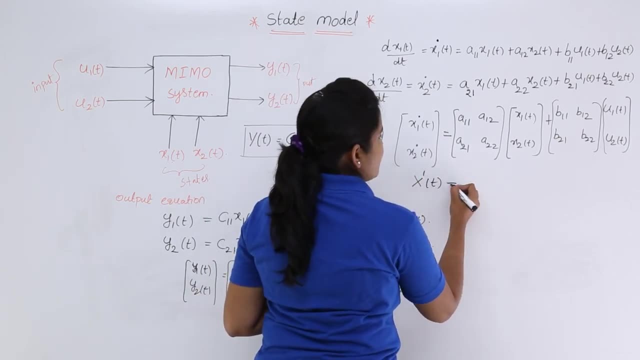 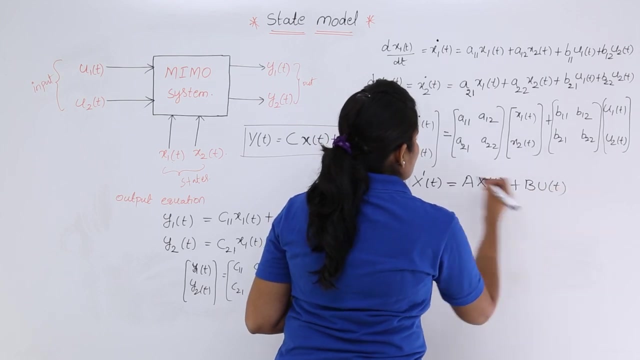 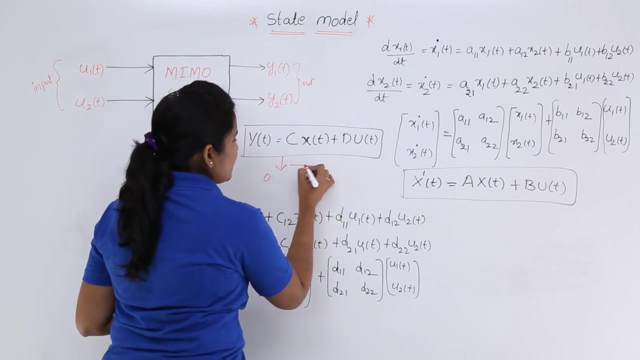 this four you will get like this: you need to write- And here this I am considering- like X dash of T is equivalent to AX of T plus B? U of T. So this is nothing but state equation and this is nothing but output equation. This is equation number one. this is output. 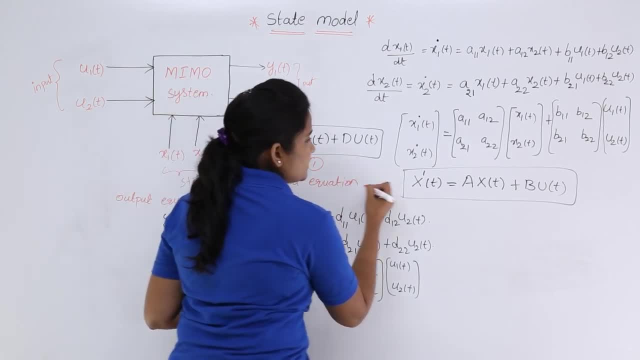 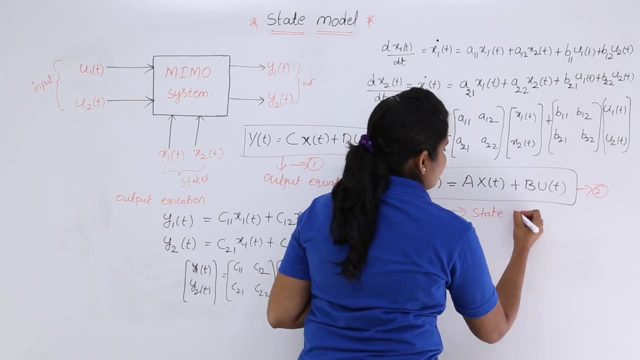 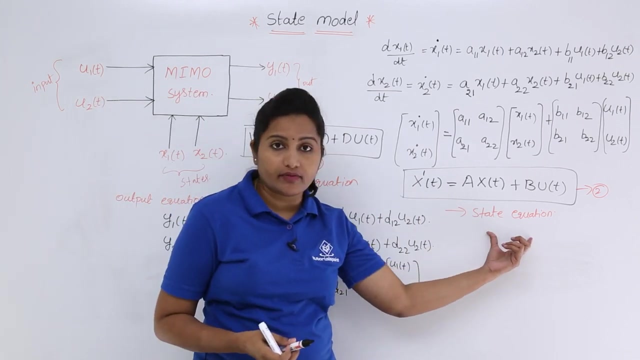 equation- Question Time: Maria Polin. Maria Polin, and this is equation number 2, this is called as state equation. We are having so many analysis based on this output equation and state equation. Please keep in mind, do not confuse when you are. 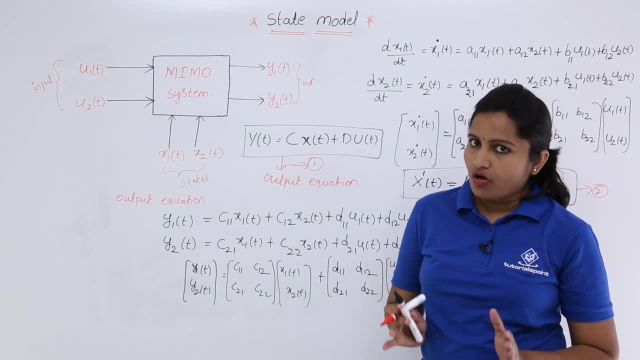 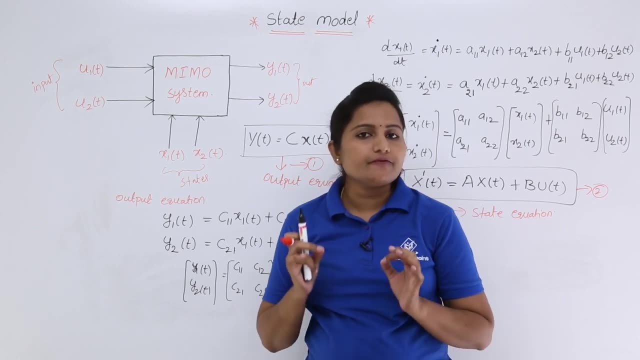 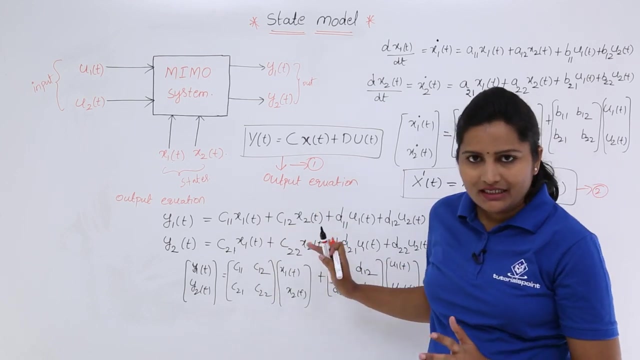 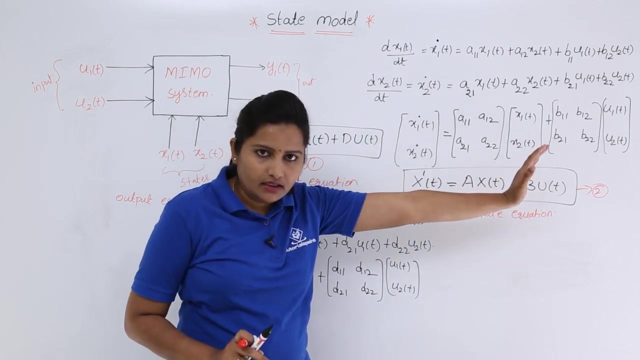 writing any output equation or state equation. we need to write with state variables and input variables only. only the difference is coefficients. For output variables I am taking cd and for state variables, writing. state equation writing. I am considering a and b as coefficients. 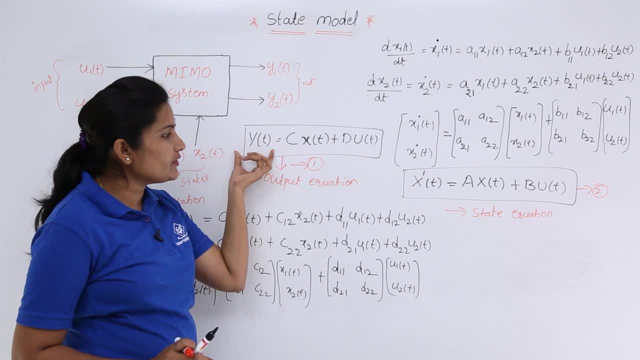 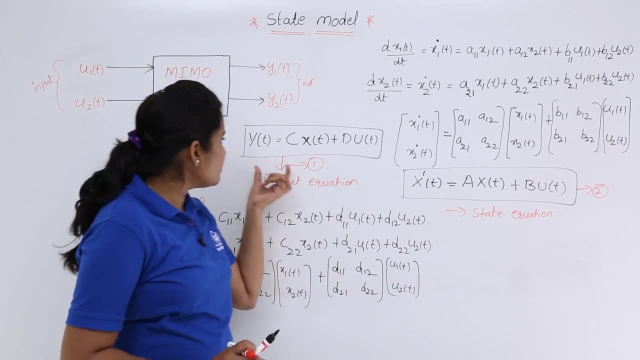 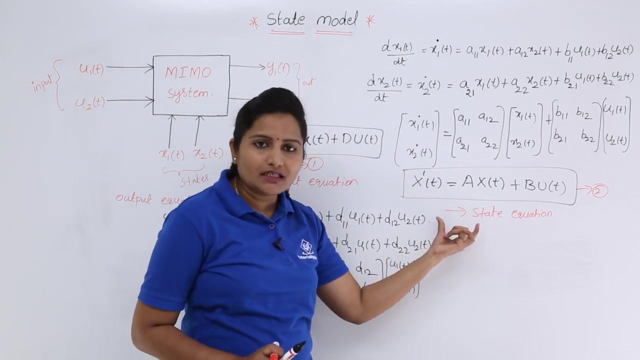 So here my output equation is: y of t is equal to. you can observe, this is output and this is state. x represents state. So this is my output equation. y of t is equivalent to c x of t plus d u of t. like that, my output state equation. 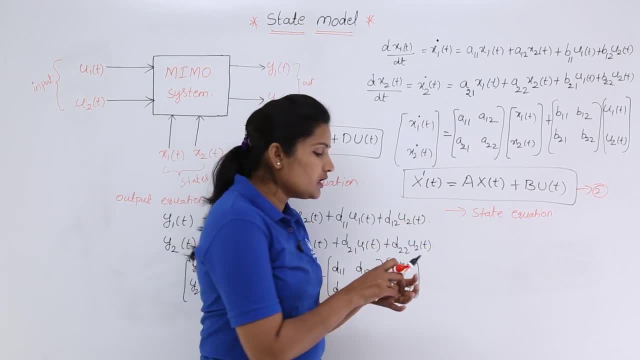 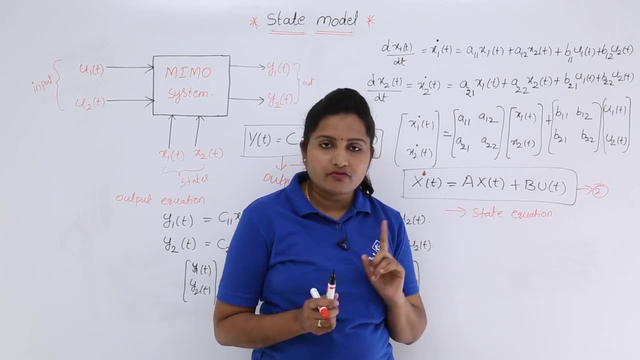 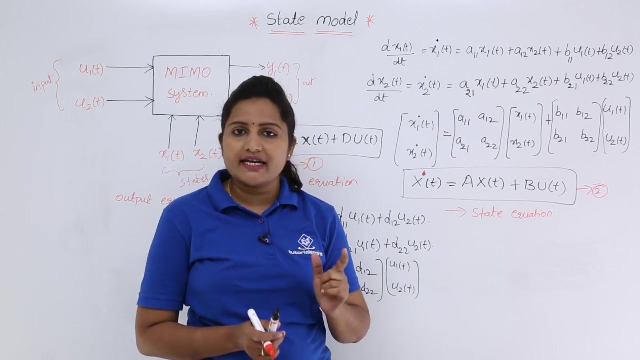 is nothing but x dash of t is equivalent to, or x dot of t is equivalent to a into x of t plus b into u of t. So equation 1 is output equation and equation 2 is state equation, both combinedly called as state model. So what is the state model means? So 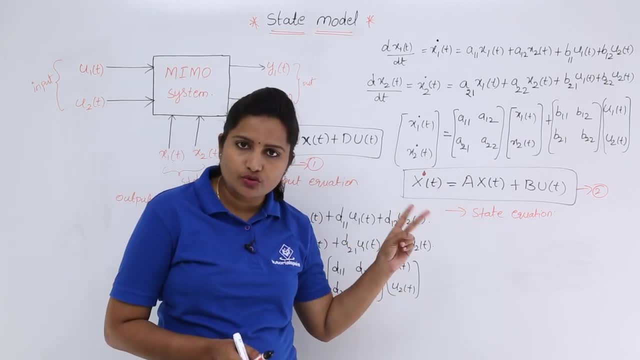 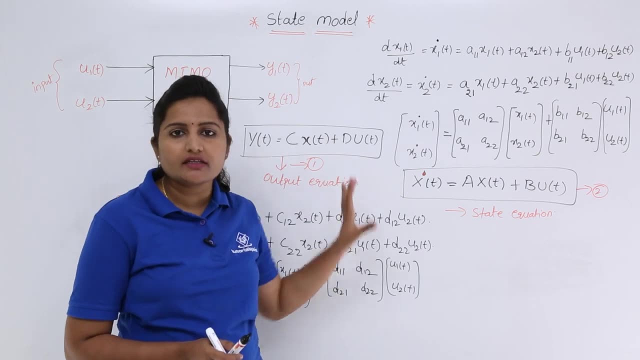 this is the output equation and this is the state equation. these two equations are nothing but state model. write the state model in the state space analysis means you need to write this derivation. So this is about state model in state space analysis. these two equations.